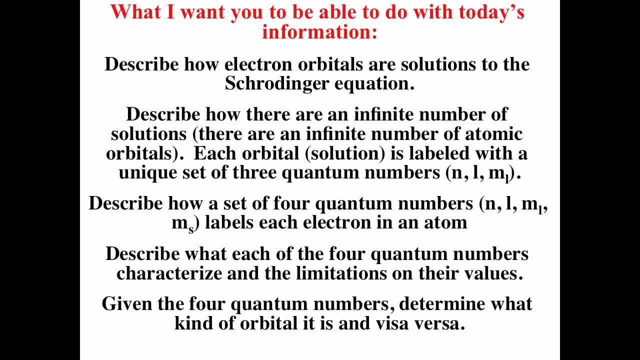 S labels each electron in an atom, And so each electron in an atom has a unique set of four quantum numbers: N, L and M, sub S, m, sub l, m, sub s. You should be able to describe what each of the four quantum numbers characterize. 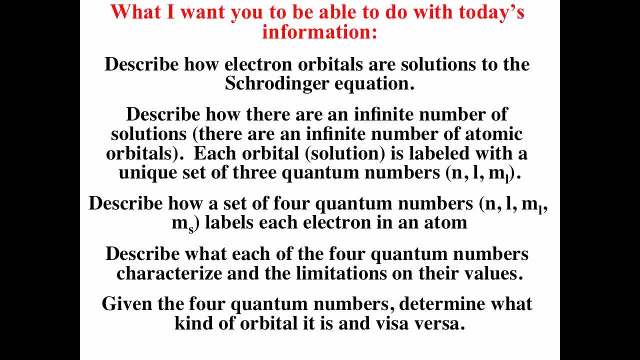 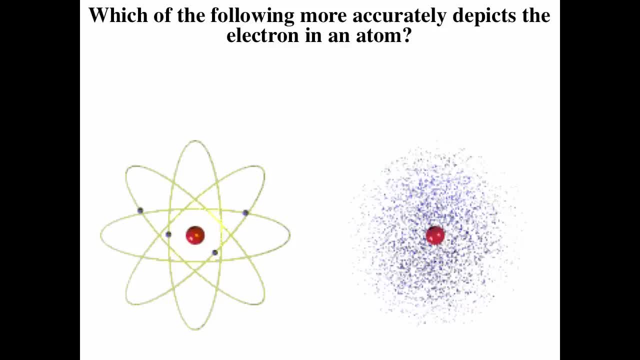 and the limitations of their values. Given the four quantum numbers, you should be able to determine what kind of orbital it is, and given an orbital, you should be able to determine what the corresponding quantum numbers are. Now, the picture on the left is a very popular enticing. 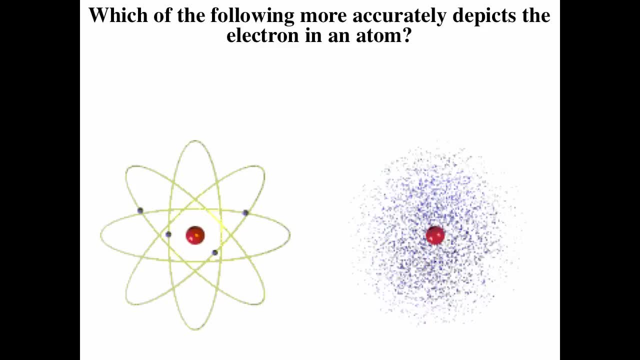 picture of electrons in an atom. It pictures the electrons orbiting the nucleus like planets orbiting the sun. It's very beautiful. I kind of think about it as the Simpsons view of the atom and unfortunately it's very, very, very, very wrong. It's very dangerous to think about. 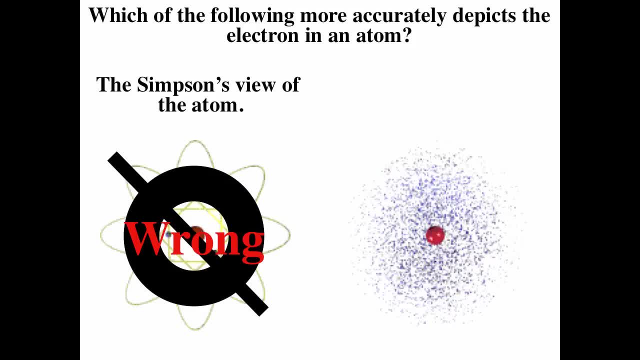 electrons in this way. Electrons have wave-like properties. They are not hard spheres. That picture shows them as hard spheres. A better, more accurate way of thinking about electrons is: you actually have electron density around the nucleus. It's smeared out. 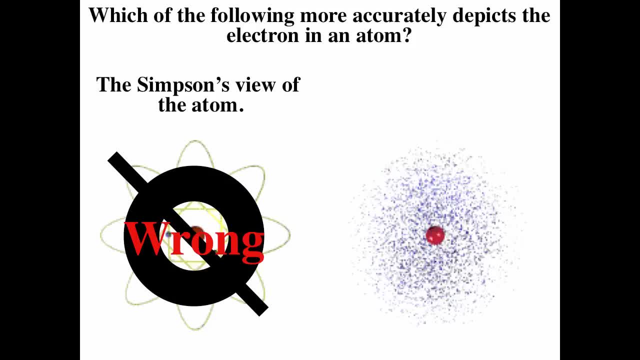 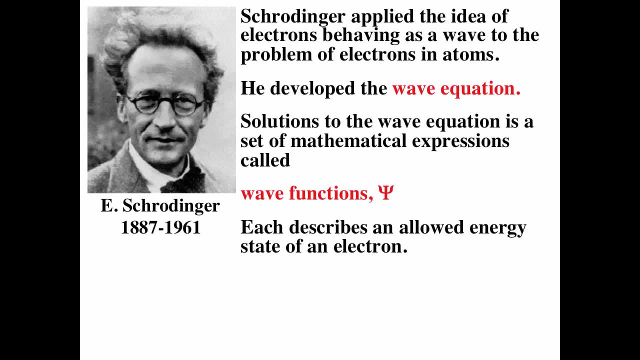 And I mentioned that to understand small things like electrons and atoms, we need to understand a little bit about quantum mechanics, And so quantum mechanics was developed between 1900 and 1925.. It was actually developed mathematically in terms of wave equations and in terms of matrices, and a year later it was 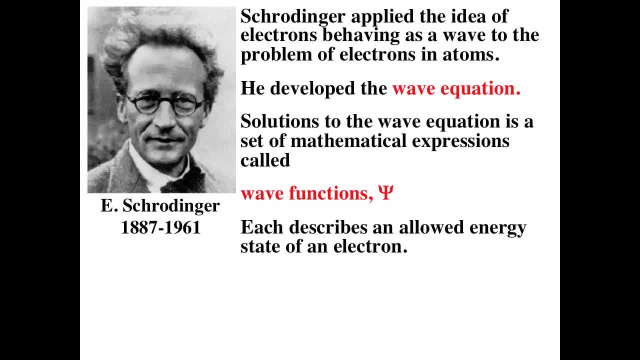 determined that those two mathematical formulations of quantum mechanics were equivalent, And so Schrodinger developed the wave equation. Heisenberg developed the matrix mechanics, And so Schrodinger had a Schrodinger equation. The solutions to the Schrodinger equation are the wave functions, which are symbolized as capital psi. 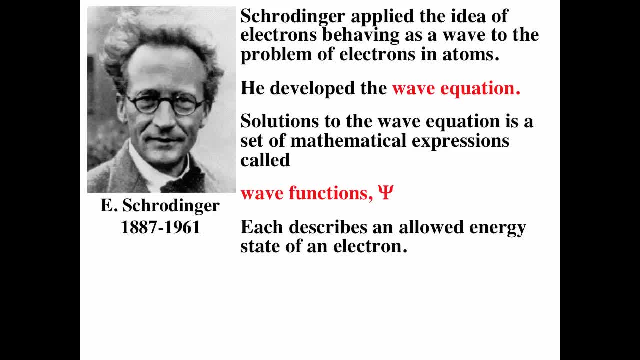 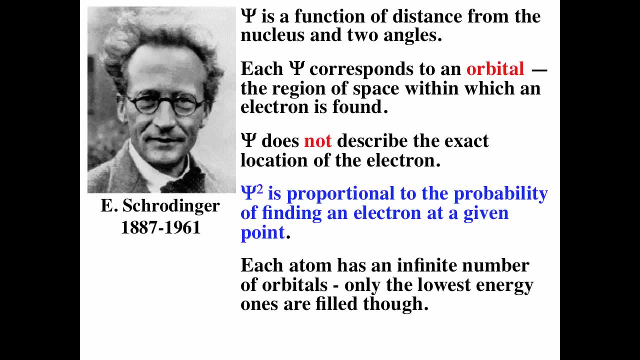 And so each wave function describes an allowed energy state of an electron, And so you can use Schrodinger's equation to solve the question of where the electrons, or what states the electrons can have in an atom. Now, psi doesn't really have a physical meaning. Psi squared is proportional to: 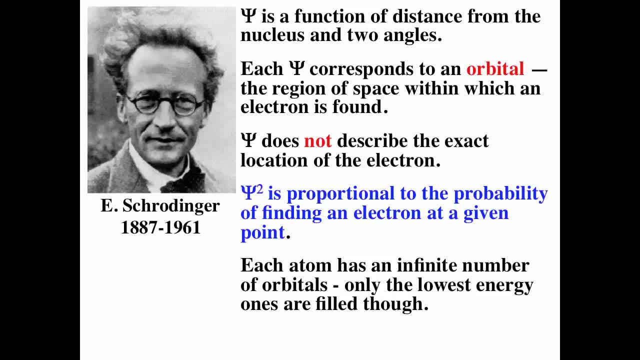 electron density of the electron around an atom. Now you can also think about psi squared as terms of proportional to the probability of the electron density of the electron around an atom. Psi squared is the probability of finding an electron at a given point. But again, I think it's better to think about. 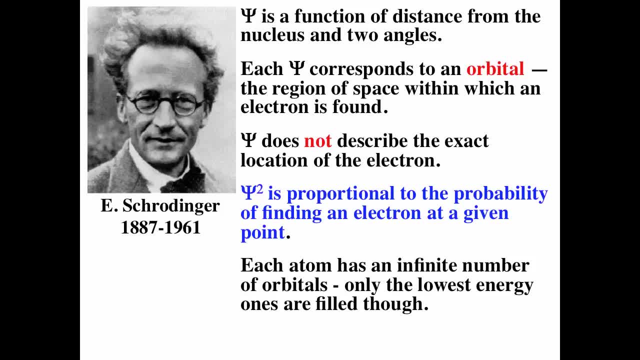 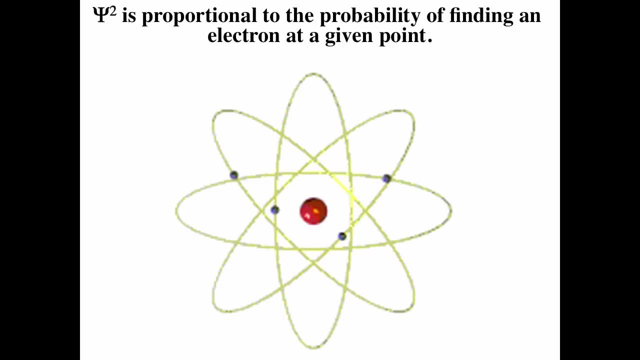 psi squared as being proportional to electron density at a given point. Now each atom again has an infinite number of orbitals. Only the lowest energy orbitals are actually filled, And so psi squared is proportional to the probability of finding an electron at a given point. or more accurately, psi squared is: 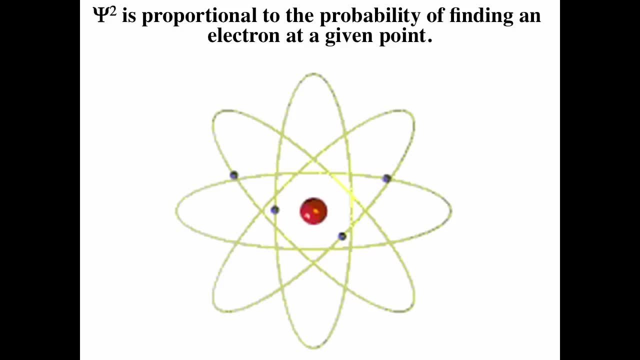 proportional to electron density at a given point. Now here's that, beautiful, enticing wrong, wrong, wrong, wrong. picture again Again. electrons do not orbit nucleus like planets orbit the sun. A familiar depiction of the atom shows electrons orbiting the nucleus like planets around the sun. 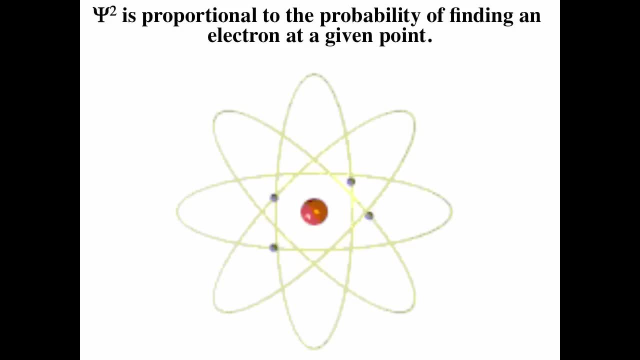 This model is neither accurate nor useful. We no longer think of electrons as orbiting the nucleus, and we cannot predict their location with accuracy. A more useful model is the quantum mechanical view of the atom, which represents the positions of electrons in terms of their probability. 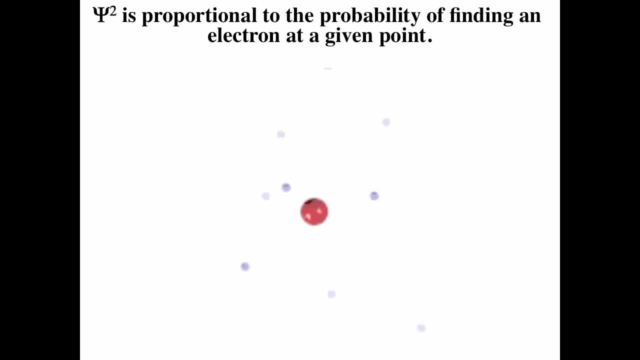 of being in a particular region around the nucleus. If we could show all positions for an electron with a specific quantized energy, the resulting picture would look something like a cloud. But again, it's probably more accurate to think about in terms of electron density. 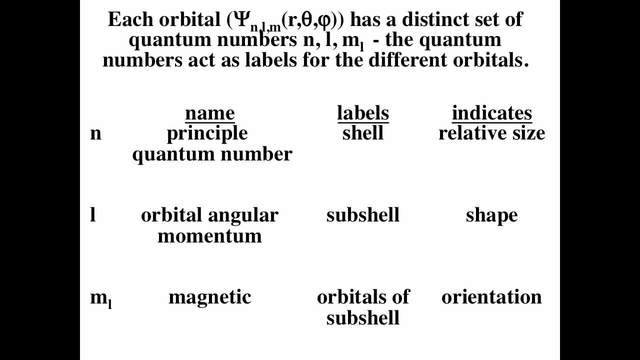 and not probability. And so I mentioned that each orbital is characterized by a distinct set of three common numbers- n, l, m, sub l- And so the common number acts as a layer of the different orbitals, and again, each orbital has a unique set of these three common. 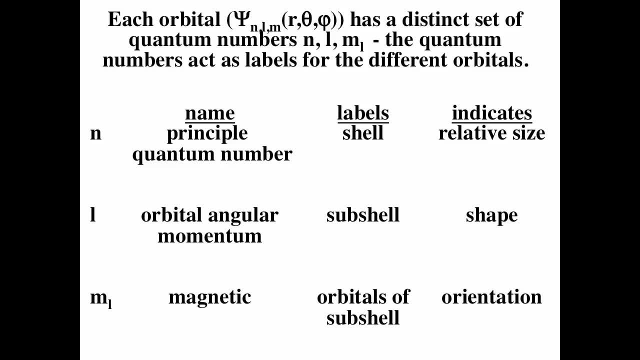 numbers. Now n is referred to as the principal quantum number. It labels a shell, And so when we talk about the first shell, we mean n equals 1,. second shell, n equals 2.. n indicates the relative size, And so the bigger the n, the bigger the orbital. l is called the azimuthal. 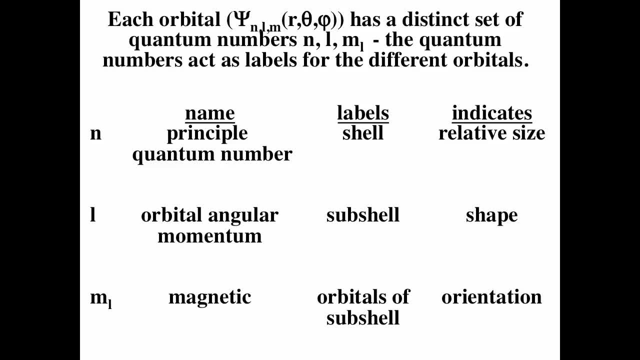 quantum number, also the orbital angular momentum. It labels the subshell, And so what we'll see is that l0 corresponds to s orbital, l1 corresponds to the p subshell And it kind of indicates the shape, And so l0 corresponds. 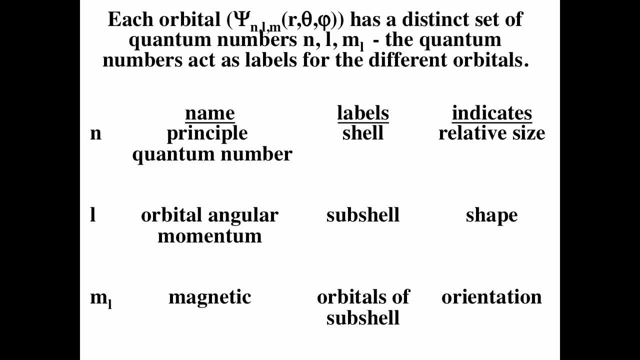 to spherical shape. l1 corresponds to a dumbbell shape, m sub l is the magnetic quantum number, It labels the orbitals of a subshell and it kind of indicates the orientation. And so l0 corresponds to s, which is spherical. 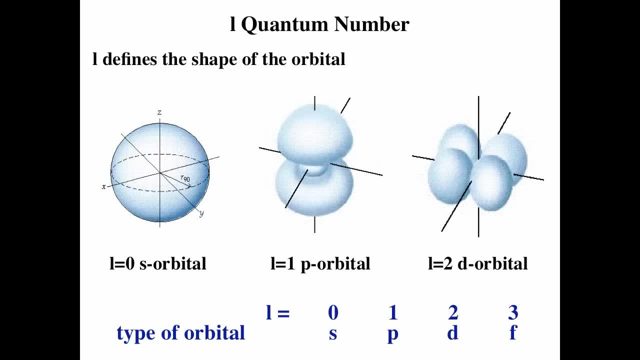 Again. l gives you the shape of the orbital. l equals 1 corresponds to p. l equals 2 corresponds to d, which is the double dumbbell shape. l equals 3 gives you an f, which is a little bit more complicated shape. 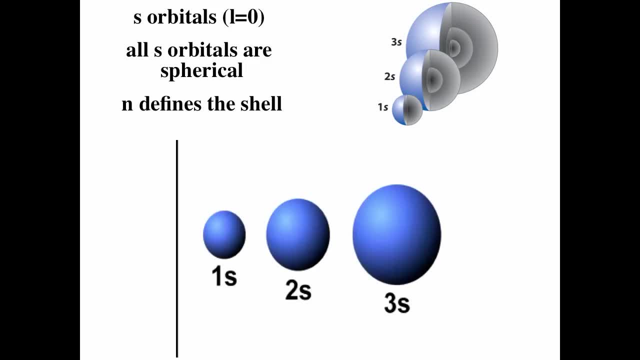 Now I mentioned that larger n, the larger the orbital, And so when we're talking about a 1s orbital, the 1 corresponds to n equals 1.. s corresponds to l equals 0.. 2s- n equals. 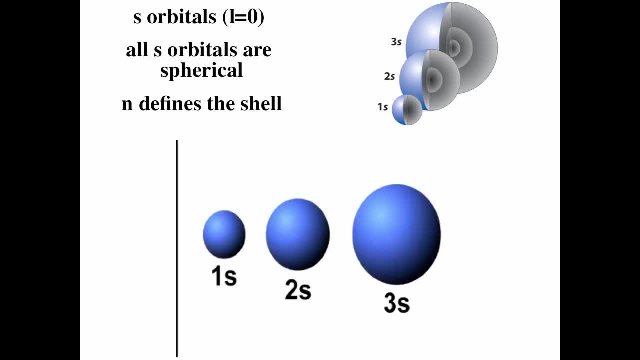 2, l equals 0.. 3s, n equals 3, l equals 0. And so bigger n, bigger the orbital, And so the 3s is larger than the 2s, which is larger than the 1s. Now, all these orbitals are s orbitals, and 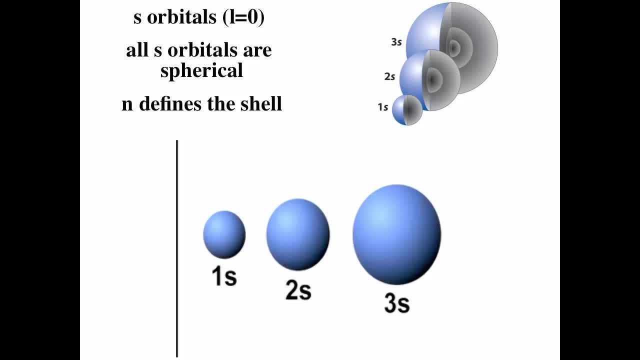 so they're all spherical. The s orbitals are all spherically symmetric, Thus contour plots connecting points of equal electron density are spheres for all values of the principle quantum number n. When n equals 1, the electron density decreases steadily with increasing distance from the nucleus. 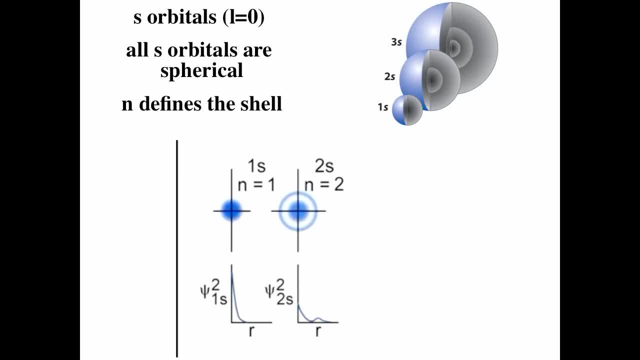 When n equals 2, the electron density goes to 0, then rises again to a new maximum. The spherical shell around the nucleus where the electron density is 0 is called a node. When n equals 3, there are two radial nodes. In summary s orbitals of differing major quantum. 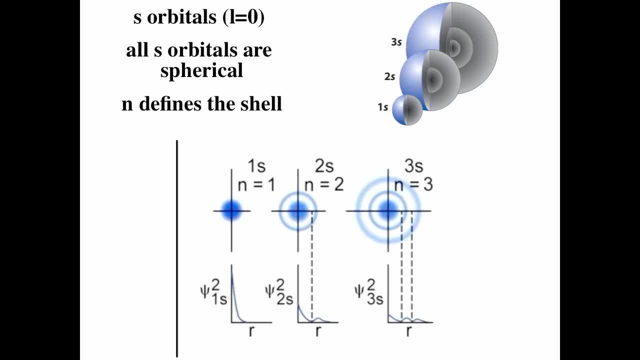 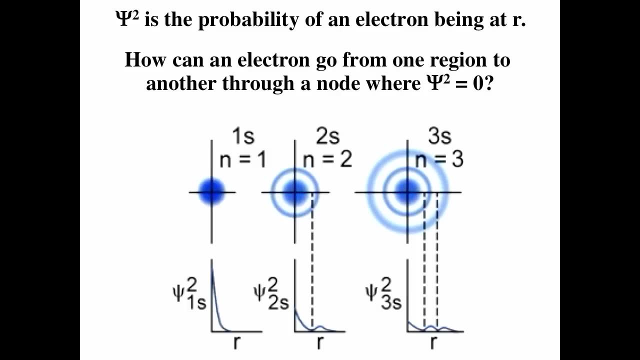 number have the same spherical shape But different. So it's kind of interesting. if you look at the bottom it shows psi squared, the electron density as a function of distance from the nucleus. And so if you look at the 2s you 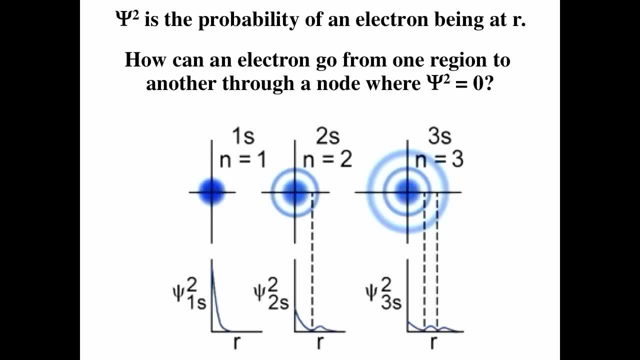 know. first, you should notice that the electron density is smeared out. okay, It's not in any one specific distance from the nucleus, but it's smeared out. And if you look at the 2s you notice that you have a node, And so at the node there's no probability of 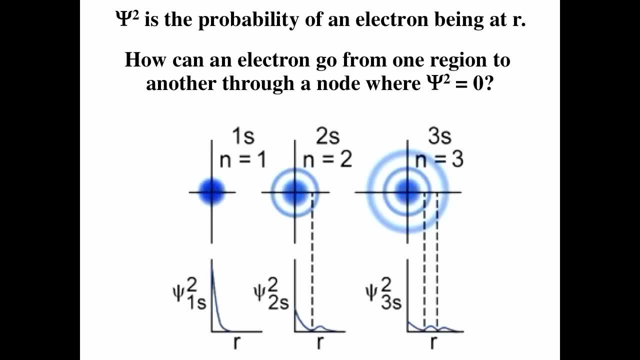 having any electron density there, And so one question you could ask yourself is: well, how can the electron go from one part of the orbital to the other part on the other side of the node, If there's absolutely no probability of it being at the node? Well again, electrons are not little particles. 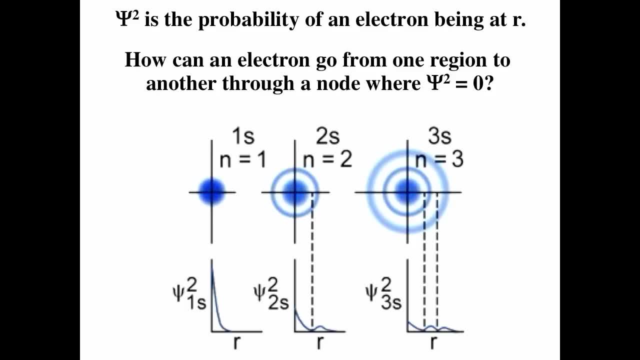 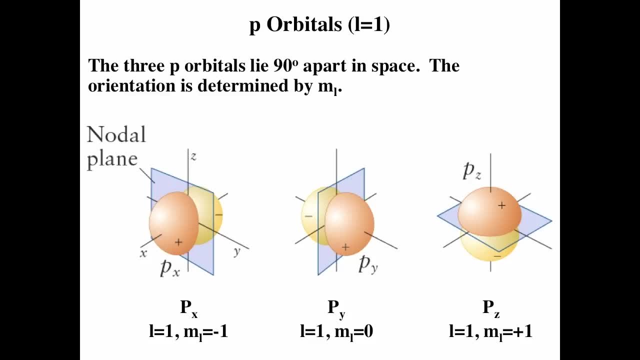 they're wave-like properties, And so s orbitals l equals 0, are spherical. p orbitals l equals 1, are in a dumbbell shape, And so you can make some井. imagine having one along the x, one along the y and one along the z, when l equals two. that 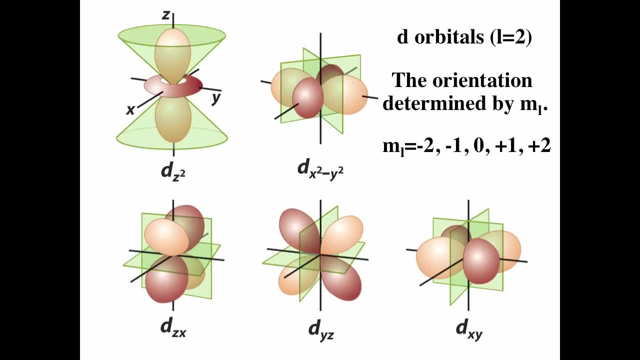 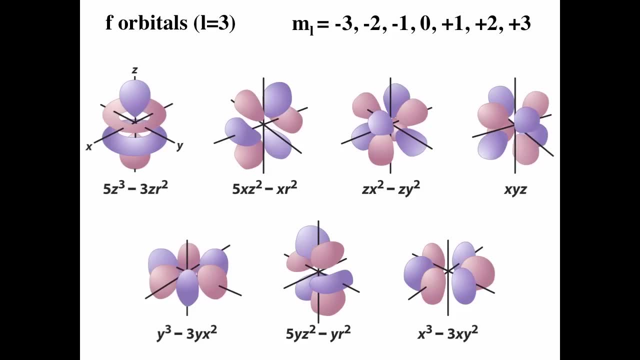 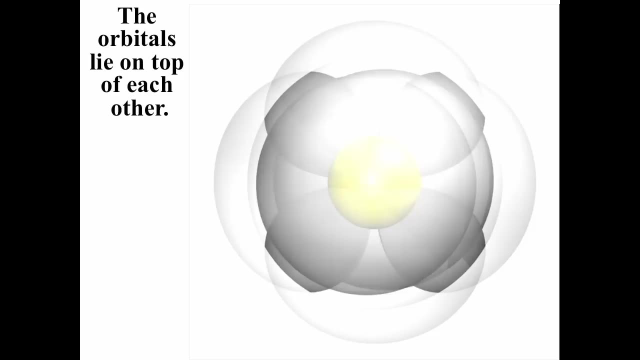 corresponds to d orbitals, and those are double dumbbell shape, except for the dz squared, which is a little bit more complex of a structure. and then l equals three is a little bit more complex, and so these orbitals all lie on top of each other, with the nucleus in the middle. now this: 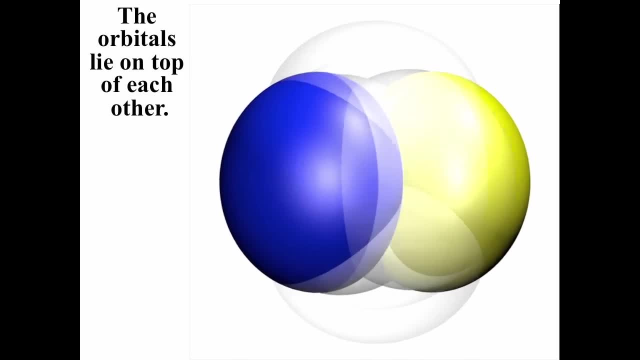 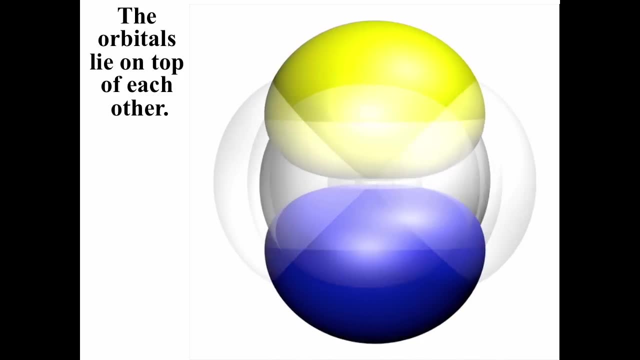 is actually a fairly decent calculation for the orbitals. what you see is that's the 1s and then the 2s, a 2p, another 2p and then the third 2p, and again remember that the electron density is actually smeared out, and so they're not on the surface of those things, but they're actually. 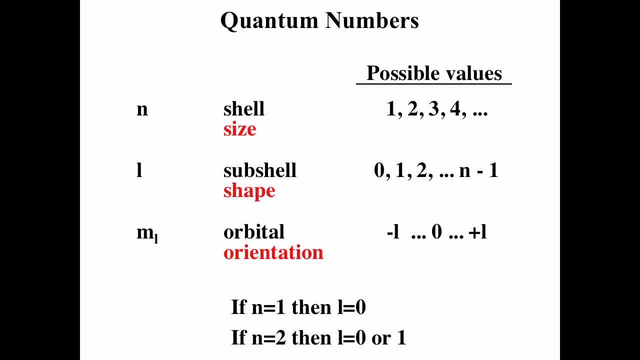 are smeared out, and so three common numbers characterize each orbital in an atom, or each orbital. an atom has a unique set of these three quantum numbers: N, L and M sub L. Now the possible values are fairly important. N can go from 1 up into an infinity. 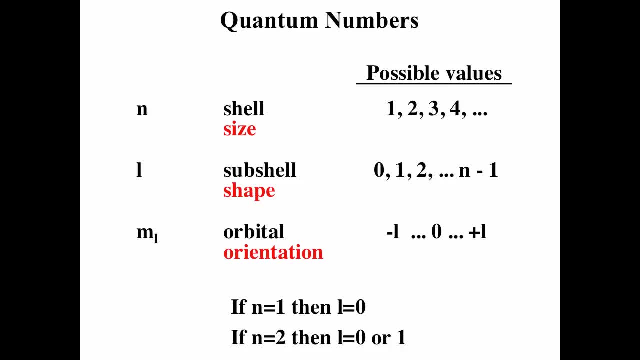 And so again, there's an infinite number of orbitals, infinite number of solutions. the Schrodinger's equation L goes from 0 to N minus 1.. And so the possible values of L depend on what shell you're in. 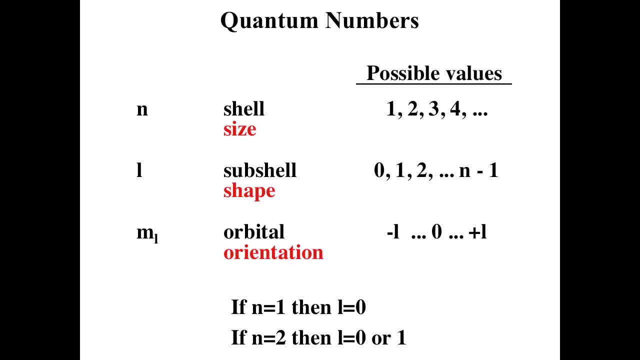 So in the first shell N equals 1, L is 0.. In the second shell, N equals 2, L can be 0 or 1.. M sub L goes from minus L through 0 to plus L, And so when L is 0, that corresponds to S. 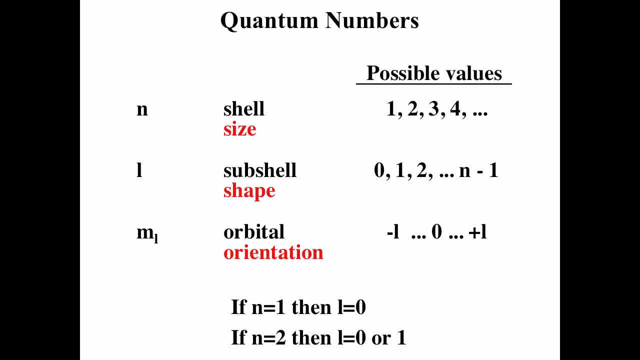 There's only one S orbital per shell. possible per shell When L equals 1, that corresponds to P. M sub L can be minus 1,, 0, or plus 1.. And so that's why there's three P orbitals per subshell. 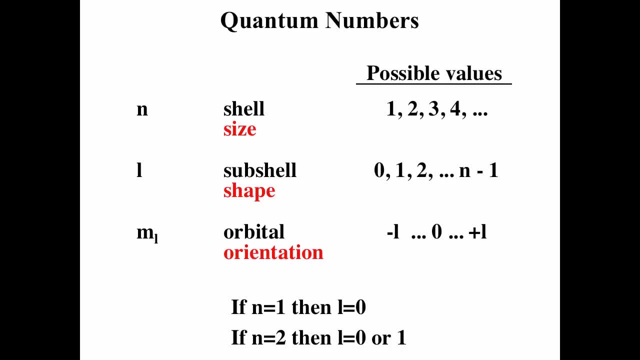 When L equals 2,, that corresponds to D. M sub L can be minus 1.. S 2, minus 1,, 0,, 1, and 2.. And so that's why there's five D orbitals per subshell. 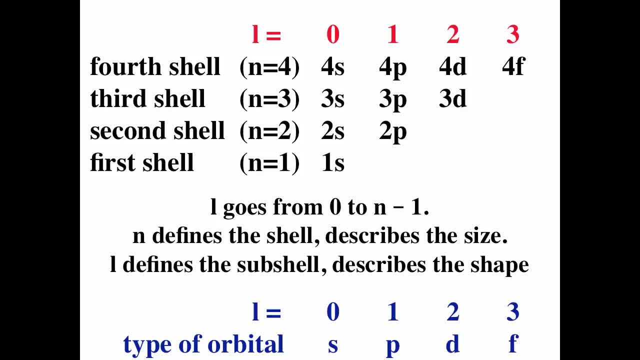 And so, if we look at the first shell, N equals 1, L can be 0.. And so that gives us just the one S. If we look at the second shell, N equals 2.. Again, N denotes the shell. 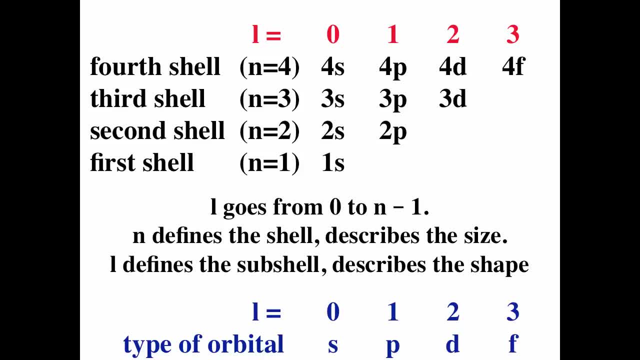 And L can be 0 and 1.. And so you have a 2S and 2P. In the third shell, N equals 3,, L can be 0,, 1, and 2.. And so you have 3S, 3P, 3D. 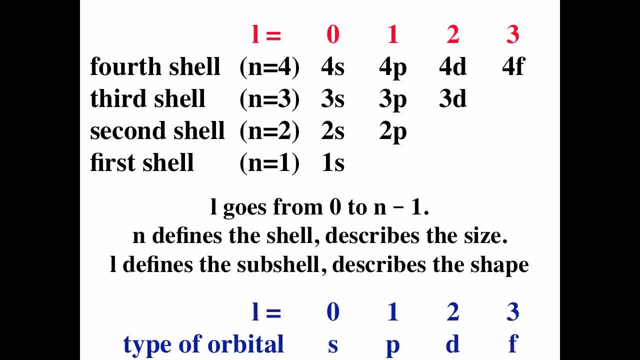 In the fourth shell, N equals 4, L can be 0,, 1,, 2S, So we're 3.. And so that corresponds to 4S, 4P, 4D and 4F. 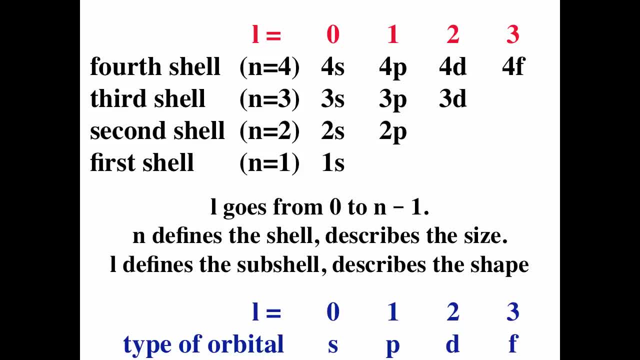 And so L goes from 0 to N minus 1.. N defines the shell, describes the size, L defines the subshell, describes the shape. And again, please remember, L0 is S, L1P, L2D and L3 is F. 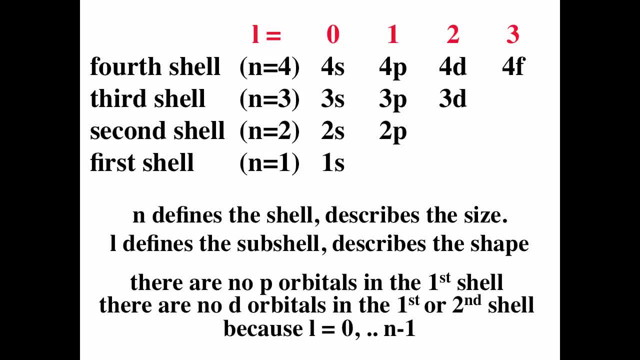 Notice that because L goes from 0 to N minus 1, there are no P orbitals in the first shell and there are no D orbitals in the first or second shell. Now M sub L goes from minus L through 0 to plus L. 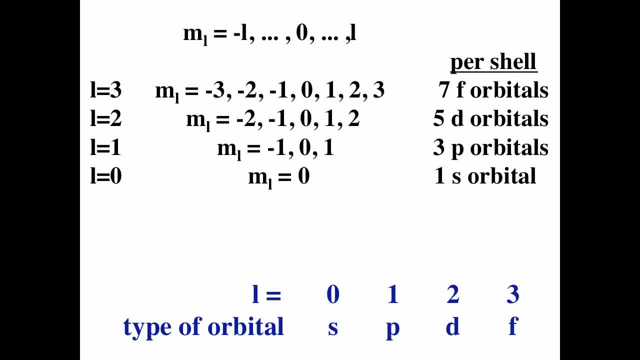 And so when L0, when you have the S orbitals, M sub L has to be 0. And so there's only one, only a single S orbital per S subshell. When L equals 1, M sub L can be minus 1,, 0, plus 1.. 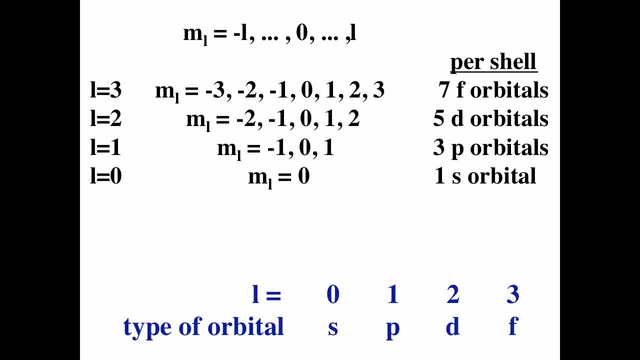 And so there's 3P orbitals per P subshell. When L equals 2, M sub L can be minus 2, minus 1,, 0,, 1, and 2. And so that gives you 5D orbitals per D subshell. 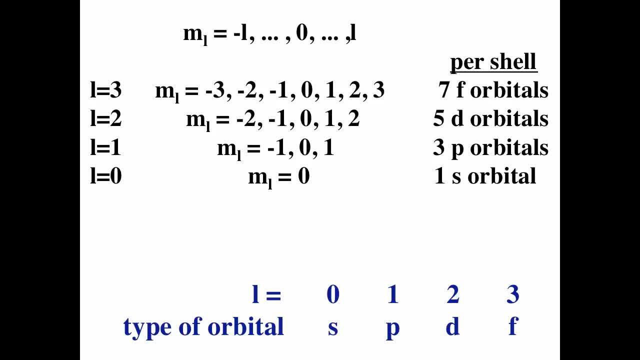 And when L equals 3, M sub L can be minus 3,, minus 2,, minus 1,, 0,, 1,, 2, and 3.. And so there's 7F orbitals per F subshell. 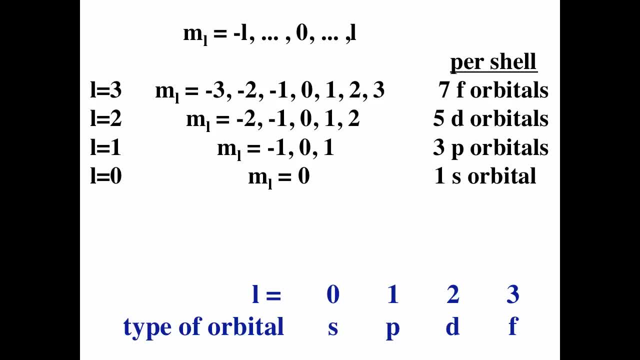 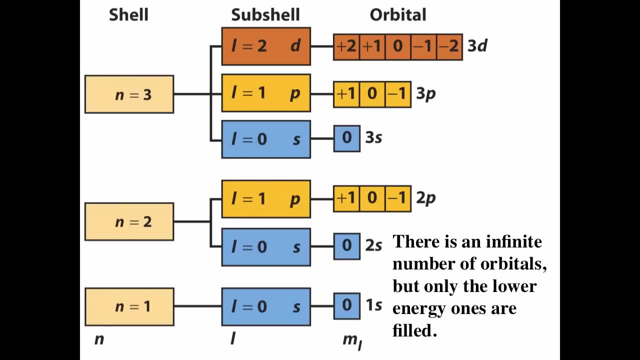 So we can depict this in a slightly different way. And so, on the bottom, we have the first shell, We just have the 1S orbital, Then we have the second shell, And so we have the 2S and the 3, 2P orbitals. 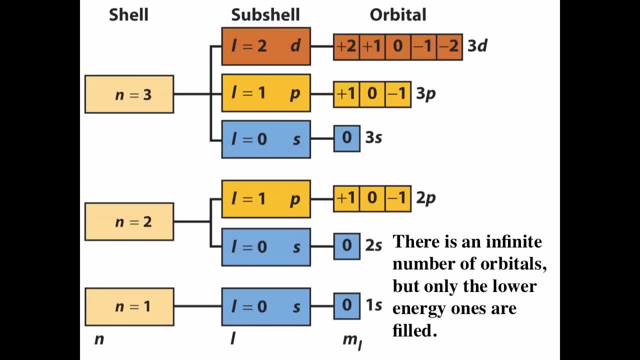 And then the third shell. we have a 3S, 3, 3Ps and 5, 3Ds, And so each orbital in the atom has a unique set of three quantum numbers: N, L and M sub L. 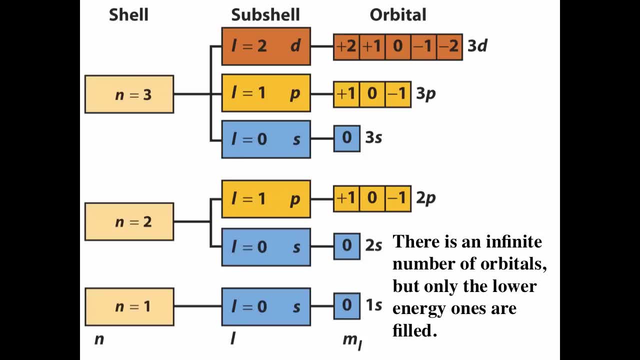 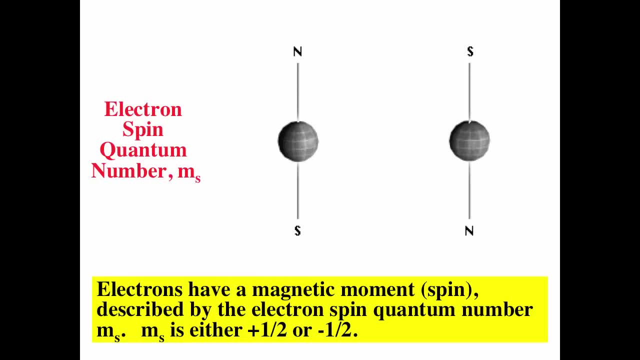 Now the electrons have a magnetic moment And when this was discovered people assumed- scientists assumed that was because the electron was spinning. You know, macroscopically or classically, sorry, when you have a spinning charge you would get a magnetic moment. 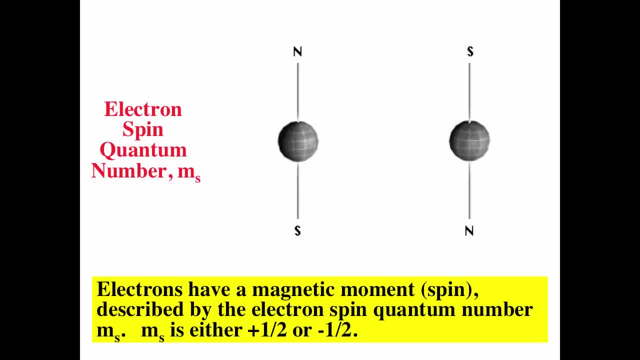 But the electron is not spinning. But unfortunately this mistake has stayed with us, And so M sub S is a spin quantum number. It denotes the relative orientation of the magnetic moment of the electron relative to a magnetic field, And it can be either plus a half or minus a half. 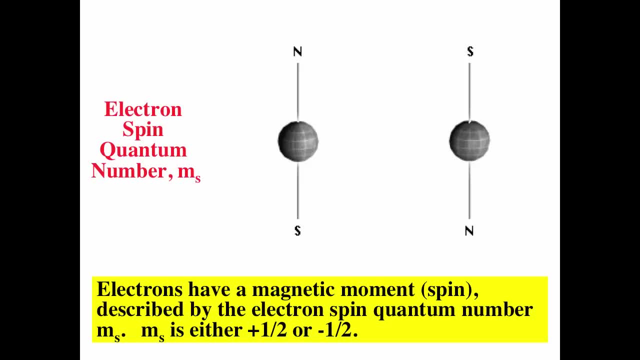 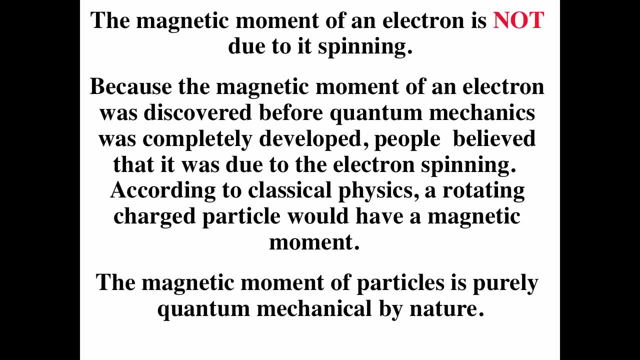 And so it's called a magnetic spin or M sub S. But again, please remember, the electron is not spinning, okay, Any spinning electric. The magnetic moment of the electron is purely quantum mechanical in nature, And so M sub S can be plus a half or minus a half. 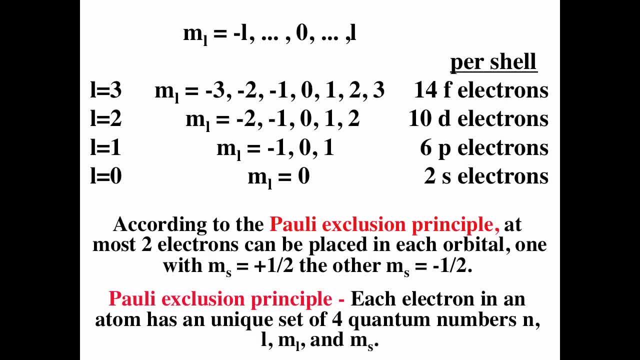 Now, because M sub S has two possible values, you can have a maximum of two electrons per orbital, And so when L is zero, that corresponds to the S orbital, M sub L has one value, So you have one S orbital per sub shell, S sub shell. 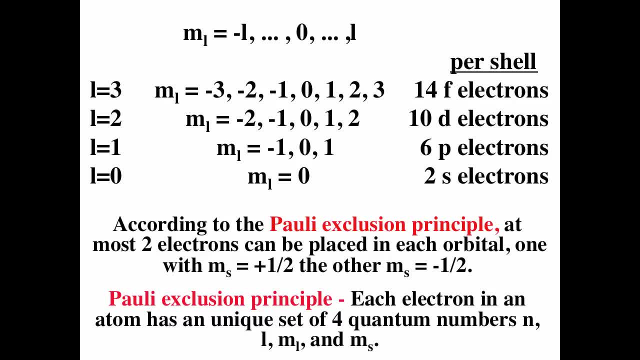 But you can have a maximum of two electrons per orbital And so that gives you two S electrons maximum per sub shell, But M sub S plus a half or minus a half, maximum of two electrons per orbital. that's the Pauli exclusion principle. 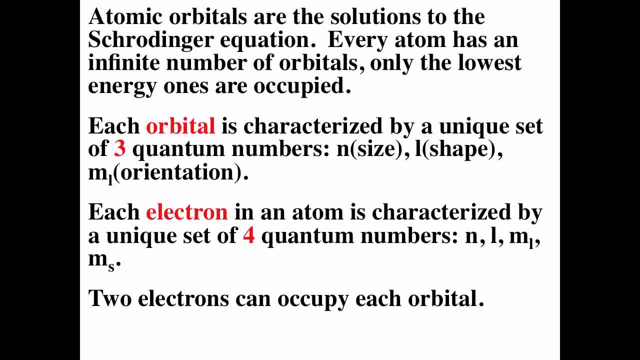 And so orbitals have a unique set. Each orbital has a unique set of three common numbers: N, L, M sub L. Each electron in an atom has a unique set of four quantum numbers: N L, M sub L and M sub S. 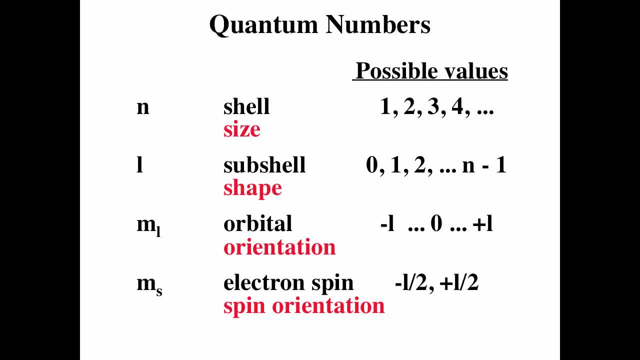 Two electrons can occupy each orbital, And so four common numbers characterize each electron. Each electron in an atom has a unique set of these four quantum numbers, And so a question you could see is how many orbitals are in the third shell? Well, a third shell means N equals three. 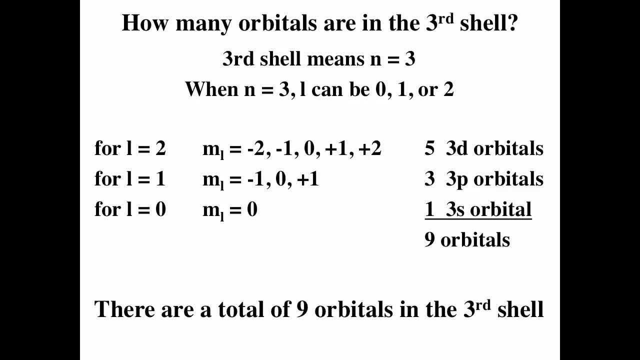 When N equals three, L can be zero, one or two, And so when L is zero, M sub L is zero. that corresponds to a single 3S orbital. When L equals one, you have minus one zero and plus one for M sub L. 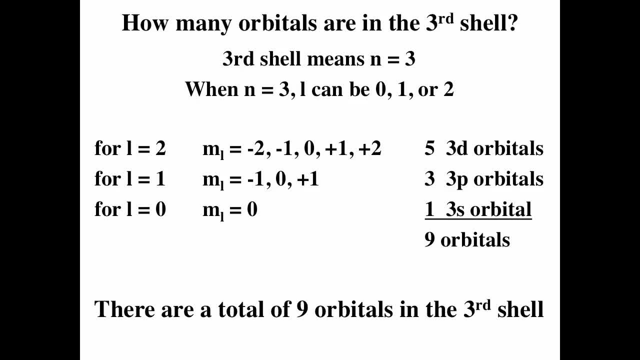 That corresponds to three 3P orbitals. When L equals two M sub L can be minus two, minus one, zero one and two. That gives you five 3D orbitals. And so five plus three plus one gives you nine orbitals. 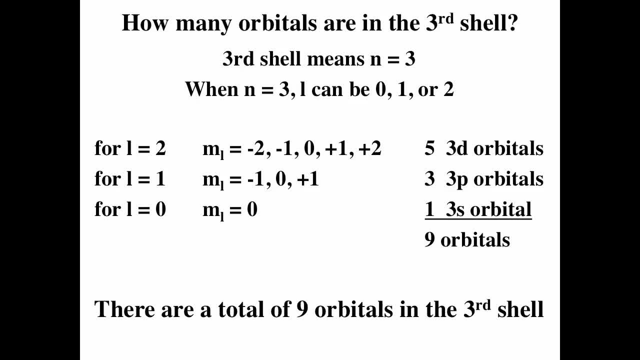 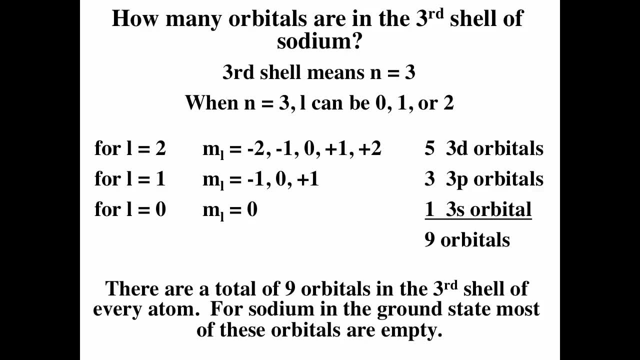 And so there are a total of nine orbitals in the third shell. Another question you could be asked is: okay, how many orbitals are in a third shell of sodium? And the answer is exactly the same: All atoms have nine orbitals in the third shell. 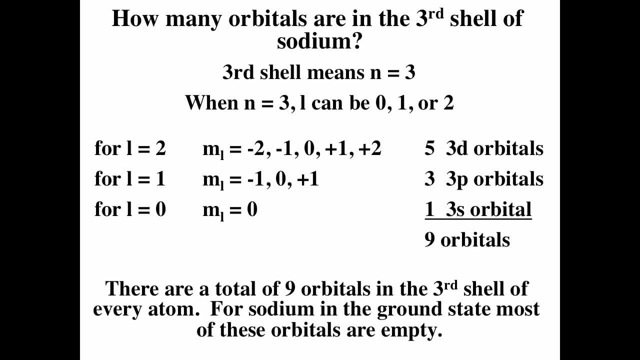 but not all these orbitals have to be filled. Okay, So there's a difference between an orbital or. an orbital is a state, it's a room, and electrons, Electrons, can occupy the orbitals, but you know, sodium has nine orbitals. 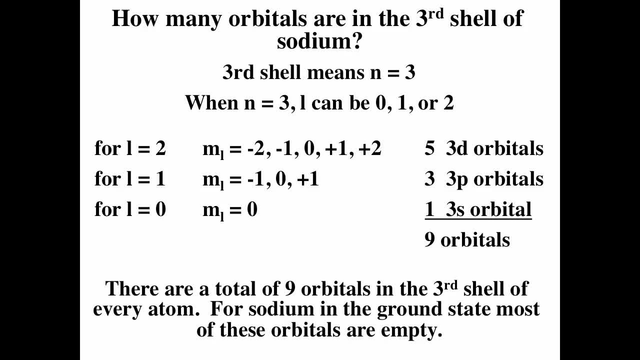 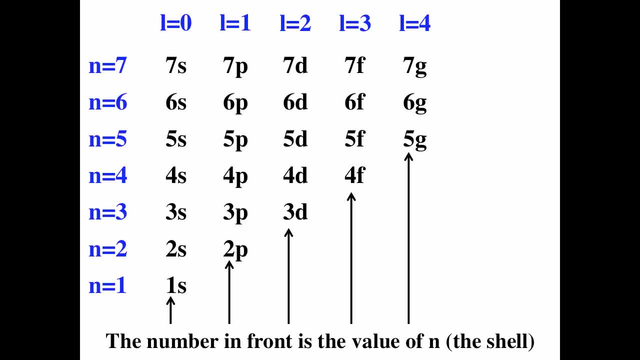 in the third shell, But actually only one orbital is occupied, And so if we take the N values on the left and the L values on top, again, remember, N is the shell, And when we talk about the 1S orbital, it means N equals one, L equals zero. 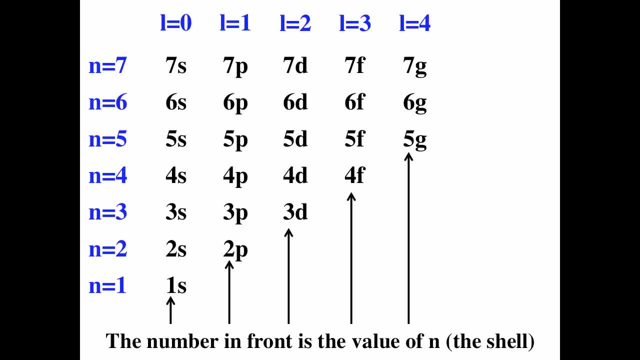 Two, P corresponds to N equals two, L equals one. Three D means N equals three, L equals two. Four F: N equals four, L equals three. Five, G: N equals five, L equals four. And so the number of front is the value of. N is the shell. 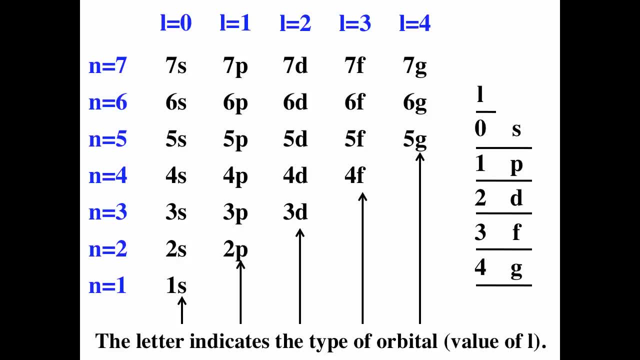 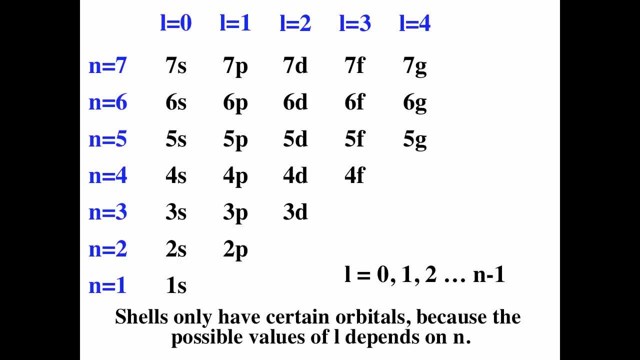 And S, P, D, F, G. well, S means L is zero, P means L1,, D, L2,, F, L3, and G is L4.. And so shells only have certain orbitals, because the possible values of L depends on N. L goes. 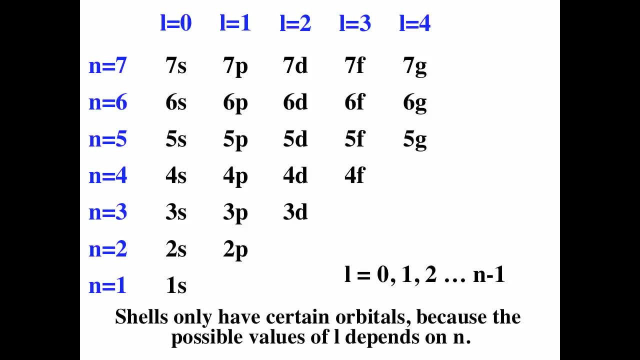 from zero up into N minus one, and that's why in the first shell you only have the 1S, In the second shell you only have the 2S, In the third shell you only have the 3S, 3P, 3D. 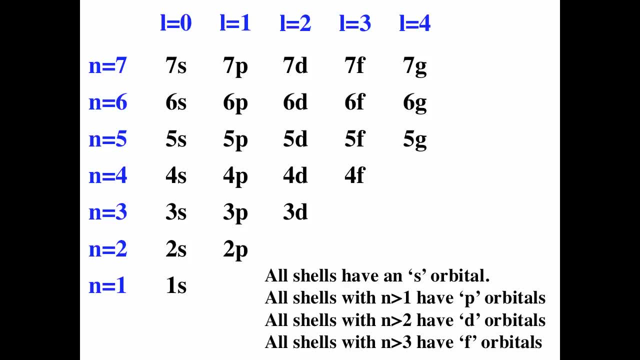 You know, all shells with N greater than one have P orbitals, All shells with N greater than two have Ds And all shells with N greater than three have F orbitals. Now I'm supposed to be able to go from minus L through zero to plus L. 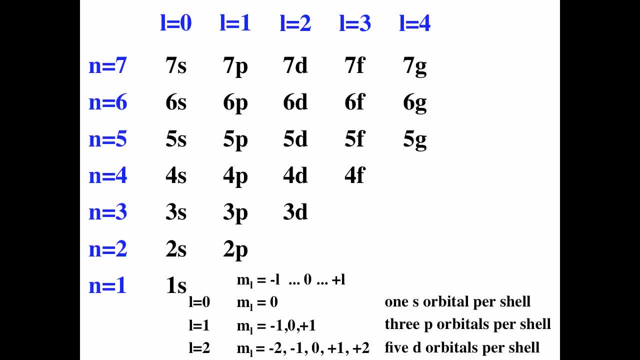 and so that's why there's only one S orbital per S subshell and three P orbitals per P subshell and five D orbitals per D subshell. Now it's kind of interesting. We'll talk about the order of filling in a later video, but in general, 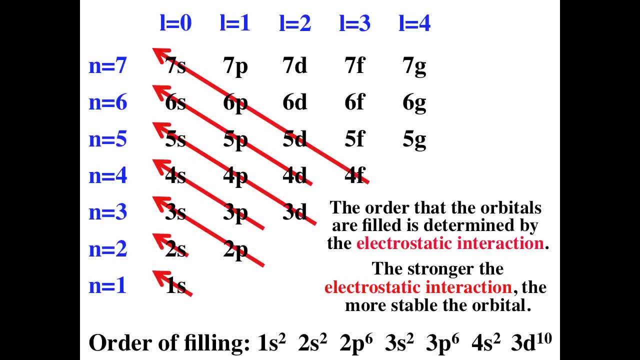 the order of filling goes 1S2, 2S2, 2P6, 3S2, 3P6, 4S2, 3D10.. The superscript is the maximum number of electrons in that subshell. 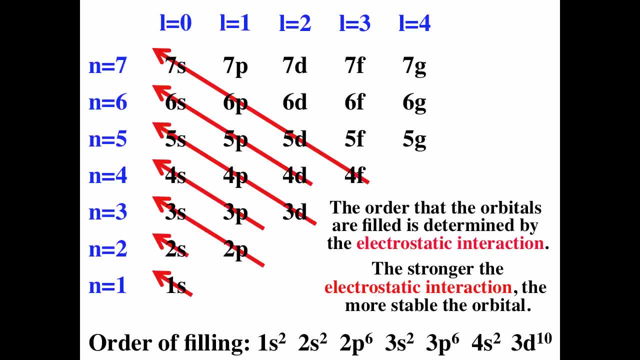 And so again: S, you have one orbital, two electrons per orbital, that gives you the two. P, you have three P orbitals per P subshell and two electrons. so three times two gives you six. And D: you have five D orbitals per D subshell. 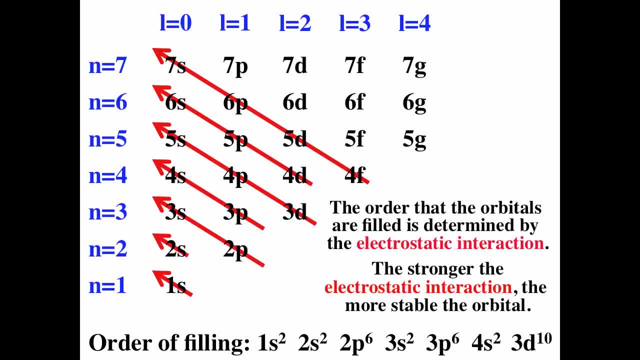 Five times two gives you that 10.. And we'll see that actually the order of filling: the lower the energy orbitals get filled first, the more stable get filled first, and it's based on the electrosec attraction between the electrons and the nucleus. 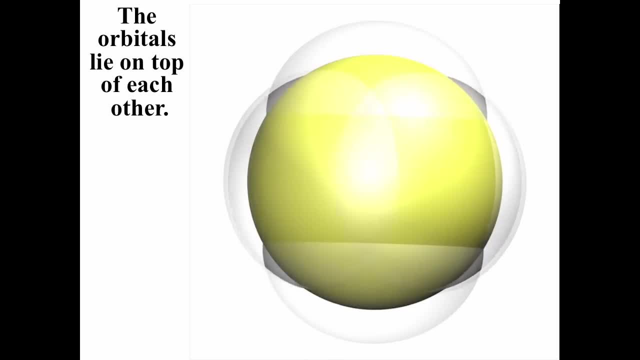 And so electrons, please remember, are not hard spheres, They're not particles. They have wave-like properties. that electrons best to think about in terms of electron density. You have the 1S, the 2S, a 2P, another 2P.